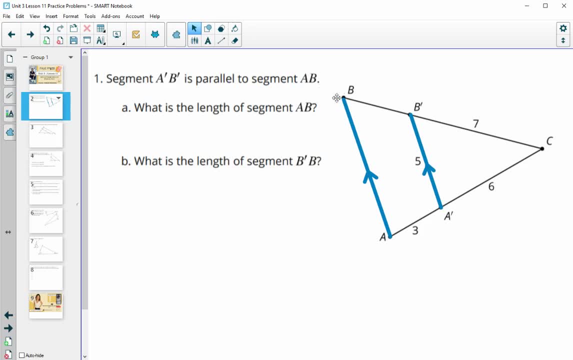 So in the lesson we learned that parallel lines will give us similar triangles. So we know that this smaller triangle here, CB'A' is similar to CBA, the original triangle, And so in this problem we're looking for the length of segment AB, which is from our original. 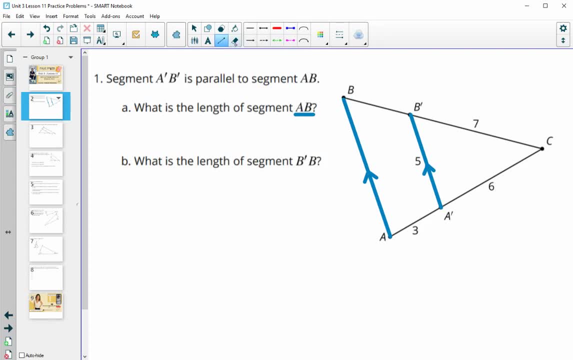 triangle. So let's take a look at setting up some proportions with the original length. So here we have the original length of AC. Okay, so the original length AC is 9, and then the image A'C is equal to 6.. This is going to help us with the length of AB. 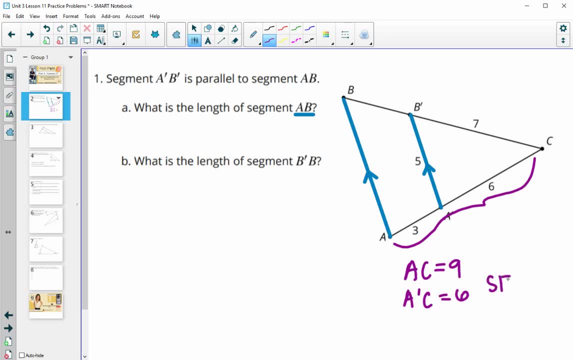 Okay, so remember that if we do scale factor it's the new amount divided by the original. So we know the scale factor connecting these two triangles is two thirds. So if you'd like to use the scale factor, you can. So in this one we have the new. 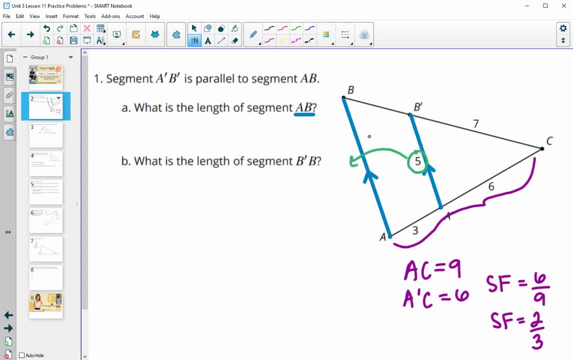 piece given. So we're going to need to divide by the scale factor to go backwards, So you would be doing 5'2". So if we use this one, we're going to get 8 coming down, 5 divided by 2 thirds. 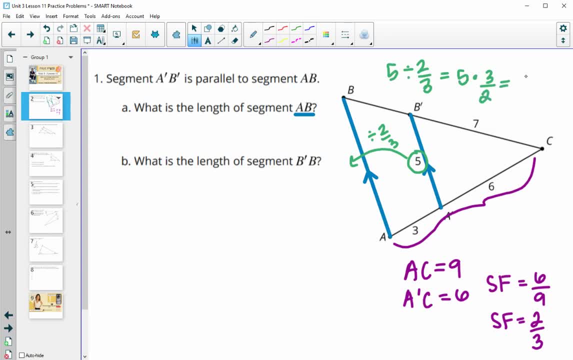 which is the same as 5, times the reciprocal. Okay, and then we get 15 on top, 2 on bottom, and 15 divided by 2 is 7.5. So then the length of AB is equal to 7.5.. So that's one way to do that. 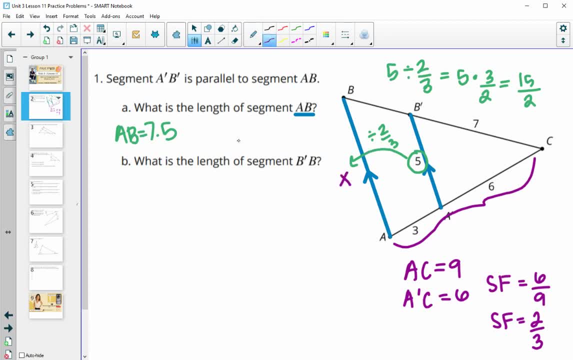 You can also set up a proportion so you can compare. So if we're looking for this side Versus its similar side in the smaller triangle of 5.. And then we can compare that to this whole length AC, which was 9 compared to its image 6.. 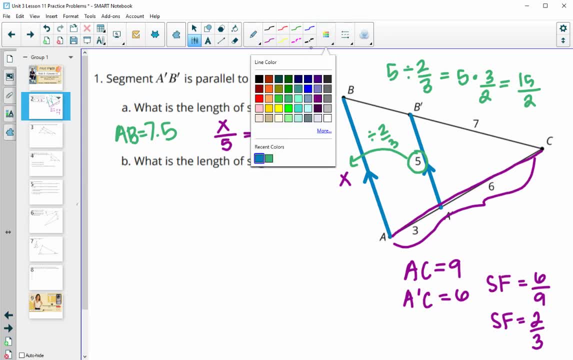 And then you can cross multiply here. So 5 times 9 is 45 divided by 6. And that gives you 7.5 as well. So looking at the original length of AB compared to the similar triangle. Now this next one asks us for the length of BB'. 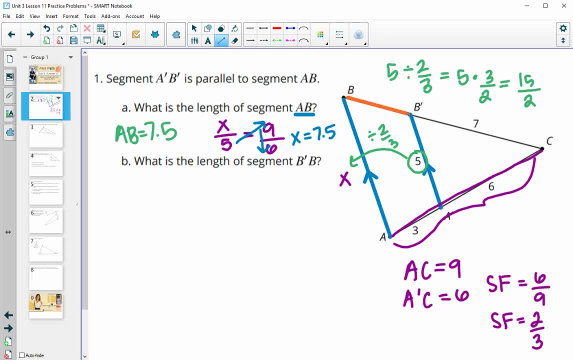 And BB' is just part of a side. It's not in one of our similar triangles. It's part of the side that's being split up by these parallel lines, And so the other thing that we learned is that these kind of split sides- here, this one compared to this one- 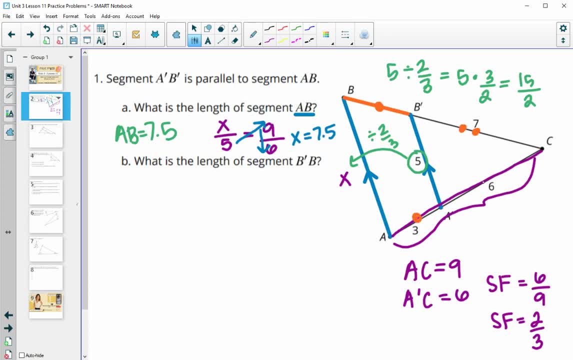 is proportional to this one compared to this one. So we know we can set up a proportion here or that they are multiplied with the same number. So if we're looking, we've got this 7.. So how does the 6 compare to the 3?? 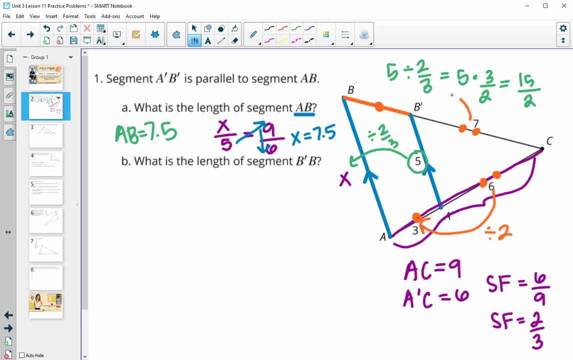 Well, we just divide by 2 to go from 6 to 3.. So we're going to do the same thing here And we can go 7 divided by 2. To get that BB' measure of 3.5.. 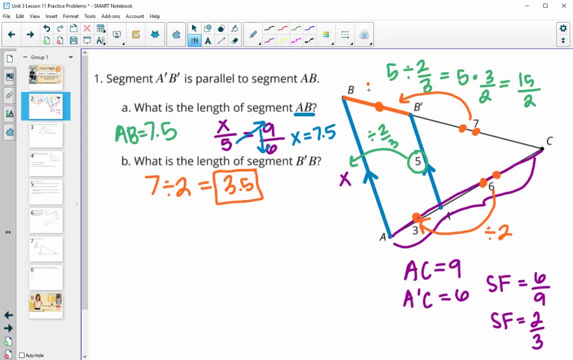 And if you like to set up proportions, you could just put a variable here and we could say Y compared to 7.. So over here I did Y compared to 7.. So I'm going to do the same thing over here: 3 compared to 6.. 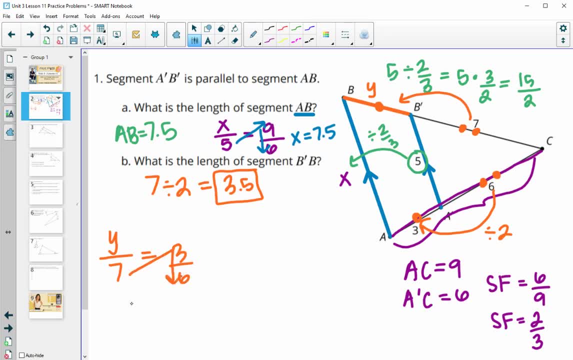 And then you could cross, multiply and divide, So 21 divided by 6. And that will give you 3.5 as well. So a couple different ways to tackle this. So I'm going to go ahead and do a couple different ways to tackle each of those problems. 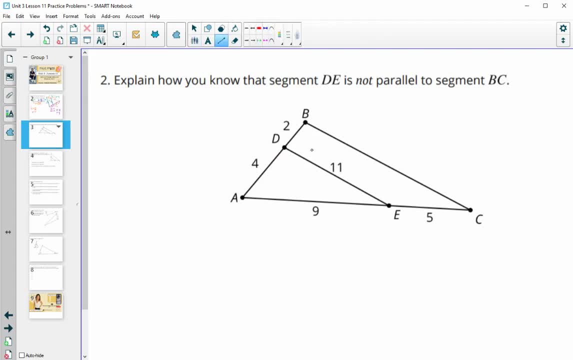 Number 2, explain how you know that DE is not parallel to BC. So if these are parallel, we know they split these sides up proportionally. So these would have to be moved by the same scale And 2 times. so this one is multiplying by 2, because 2 times 2 is 4.. 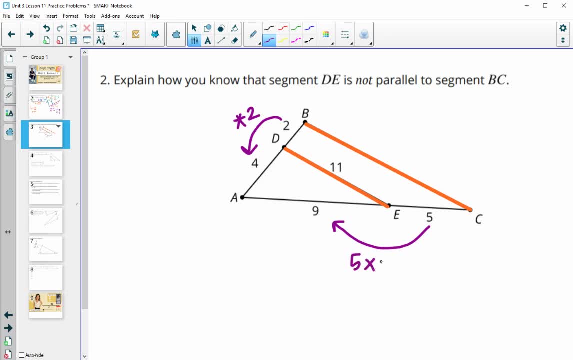 Well, 5 times 2 is not equal to 9.. OK, so 5 times 2 does not equal 9.. So these sides are not proportional, meaning they would not be parallel. So you could show your work something like this: 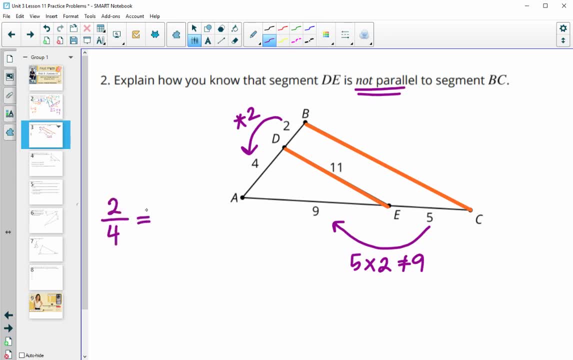 You could also show, when I compare 2 to 4, that that does not equal 5 compared to 9.. Because 2 divided by 4 is 0.5 and 5 divided by 9 is 0.55, repeating, So those are not equal. 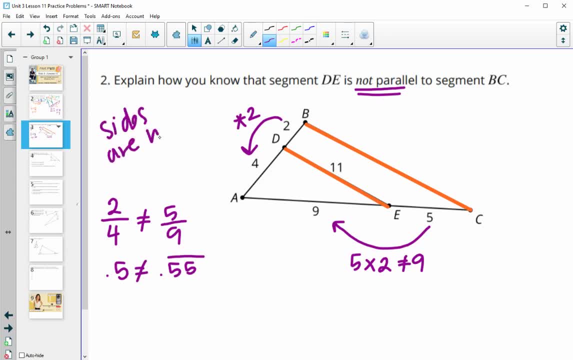 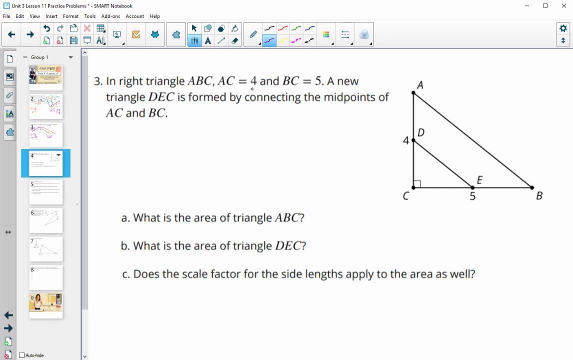 So this means the sides are not proportional And therefore not equal, or sorry, not parallel. Number 3, in a right triangle, AC is equal to 4, BC is equal to 5.. So kind of these longer segments here. 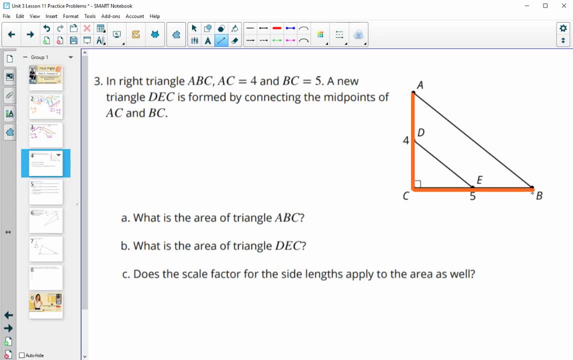 OK, the whole segment here is 4.. The whole segment here is 5.. And then it says we get this new triangle, OK, this smaller triangle down here. They're formed by connecting the midpoints, So this point D is right in the middle. 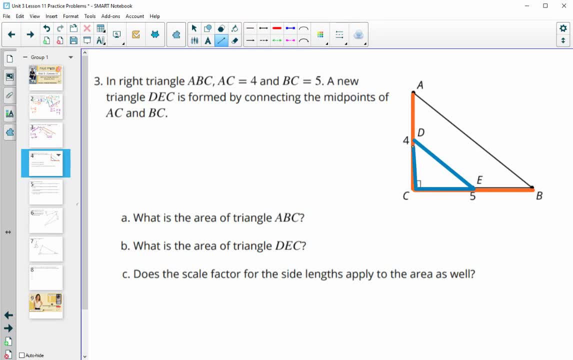 And this point E is right in the middle to get this smaller triangle, And so, since it's the midpoint, we can figure out the length of those sides by just dividing the original by 2.. So 4 divided by 2 gives us 2 for this, 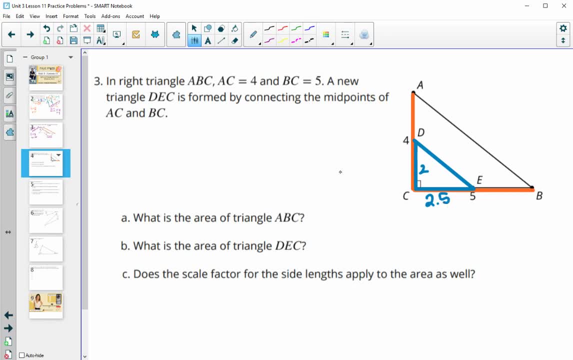 And 5 divided by 2 gives us 2.5 here. And so this one's asking: what's the area of triangle? A ABC, that larger one? And remember, area formula for a triangle is, you do, base times, height divided by 2.. 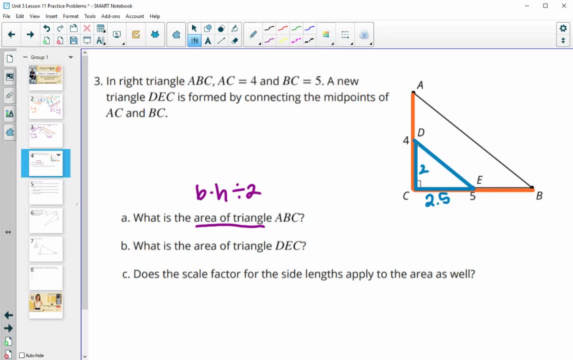 So we're going to take, and the base and the height always connect with a right angle. So this 4 and 5 are our base and height. So we'll do 4 times 5, which is 20.. And then we'll divide it by 2,, which gives us 10 units squared for the area of the orange triangle. 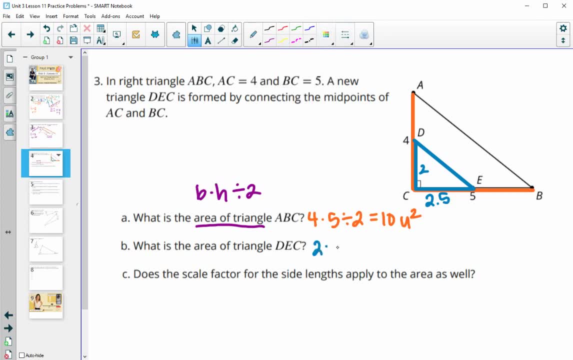 Then for the blue triangle, We'll: OK. So we'll again multiply the base, which is 2, and the height, 2.5.. OK, So 2 and 2.5 are your base and height, And then divide by 2.. 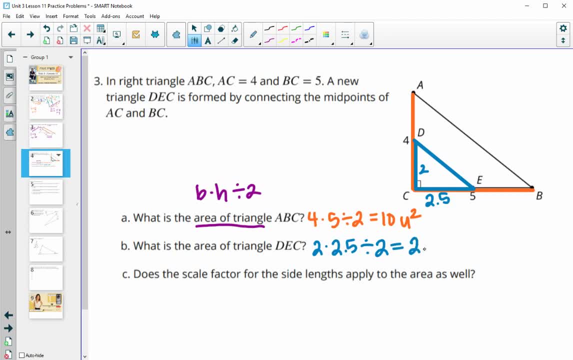 So 2 times 2.5 is 5. divided by 2 is 2.5 units squared for that blue triangles area. Then part C asks us: is the scale factor for the side lengths? Does that apply to the area as well? 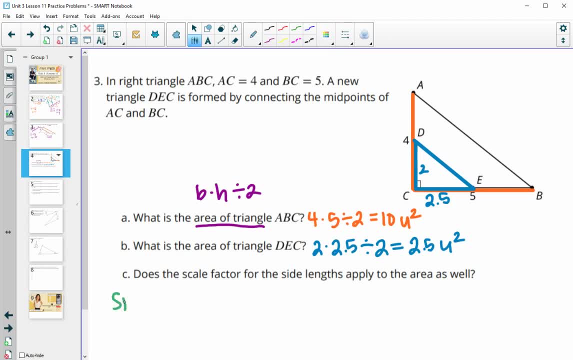 So when we look at the side Length scale factor, We know we split it at the midpoint. OK, So we know that the scale factor was one half. You can also, if you didn't realize that you could, take the new measurement 2 divided by the original measurement 4.. 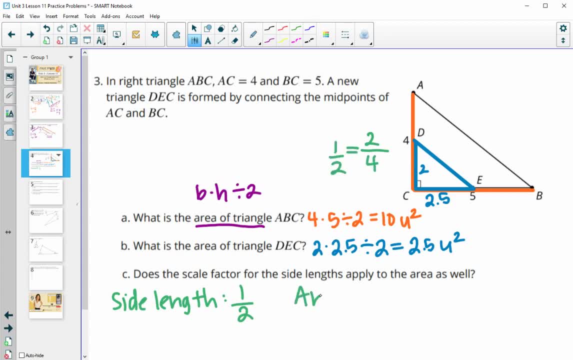 And that's where that scale factor is coming from. So now our area factor. So again, compare the new area, which is 2.5, to the original area, which was 10.. So again, compare the new area, which is 2.5, to the original area, which was 10.. 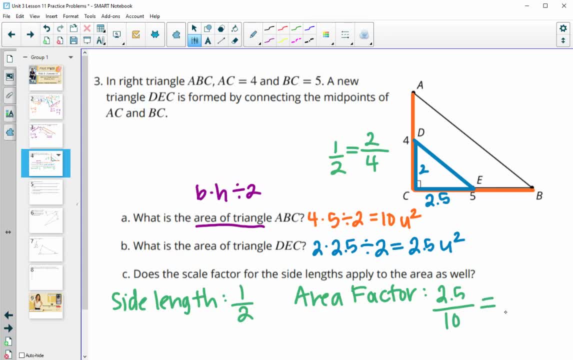 So again, compare the new area, which is 2.5, to the original area, which was 10.. OK, And this simplifies. If you wanted to look at it as a decimal, it simplifies to 0.25 and that's a fraction of one fourth. 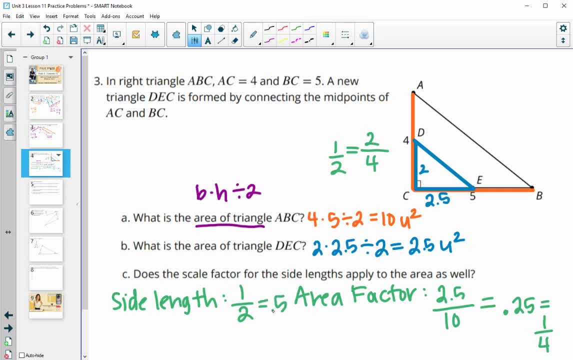 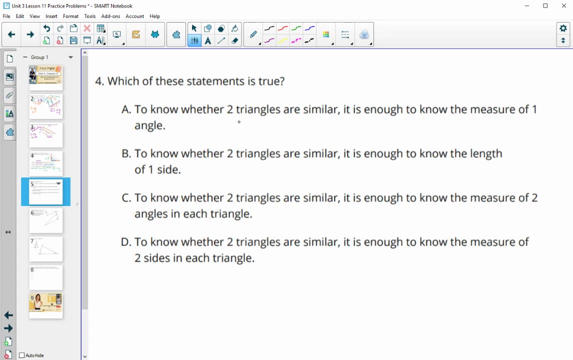 And so this side length factor was one half or a decimal of 0.5. So they do not match. So this: the side length scale factor and the area factor are not the same. Number four: which of these statements is true? So in order to know that two triangles are similar, it is enough information. 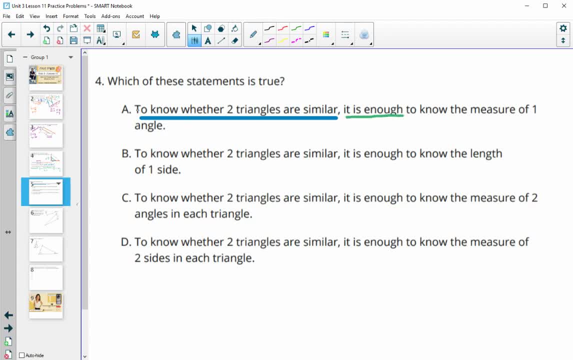 So it is enough to know the measure of one angle. That is not true. So when we're looking at how, what we need in order to prove triangles are similar, Remember we needed two angles, So angle angle similarity. We needed all three sides to be proportional. 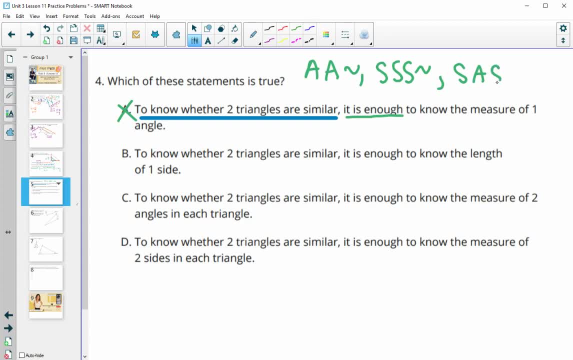 OK, Or we needed to know two sides were proportional And the angle between them. So these are the options that we have, So that first one is not happening. to know Two triangles are similar, It is enough to know the length of one side. 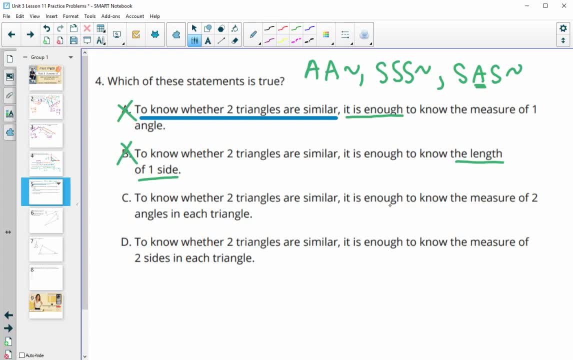 No, To know two triangles are similar, It is enough to know the measure of two angles in each triangle. Yes, If we knew two angles, we could make sure what the third one was and we could see if They match with the other triangle. 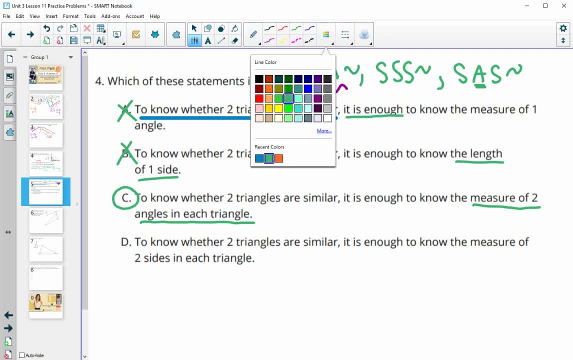 So that would definitely be enough. And then this final one: to know whether two triangles are similar. It's enough to know the measure of two sides in each triangle, And that is not true. If we have two sides, we must also know the angles, the angle between the sides. 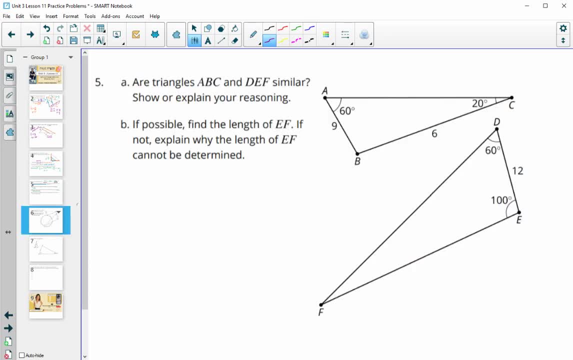 So we can check if it's the same, All right. Number five says that that are the two triangles here. Similar, show or explain your reason. So when we look here, hopefully those angles stick out to you that they're giving us two angles. 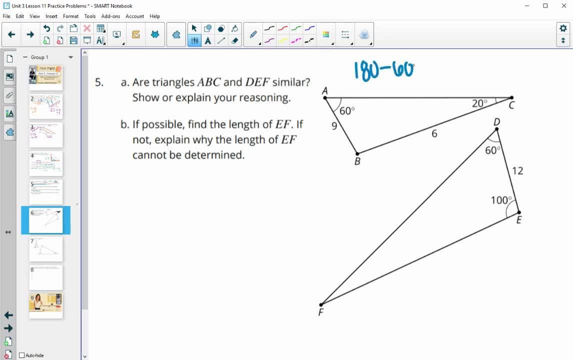 So in this first one we can do 180 minus 60 minus 20. And that gives us 100 degrees for this missing angle. And then you can see that that matches with the 100, and they also have a 60 in common. 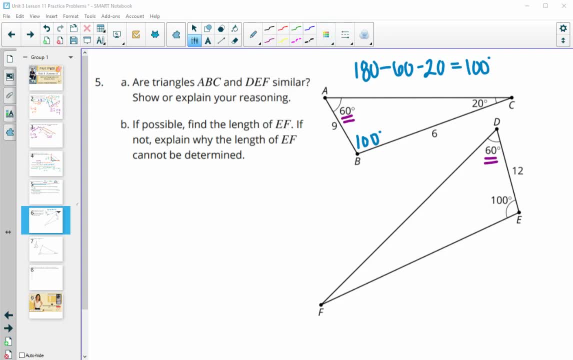 So these are. They're going to be similar by angle angle, And then we also know that this angle here is going to be equal to the other angle of 20.. So now this wants us To all. we should probably say by angle angle similarity here. 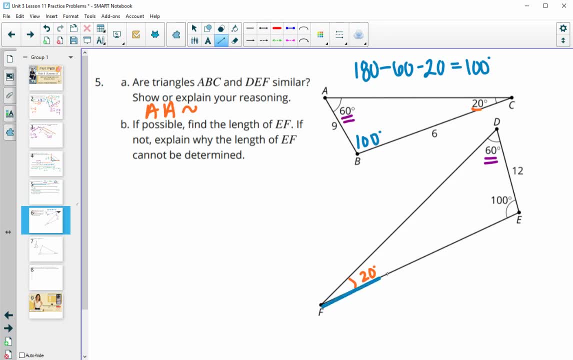 Then it wants us, if possible, to find the length of segment EF. So here's the side length they want us to find. So this side length is Similar to the one that connects the 100 and the 20 degree angle in triangle ABC. 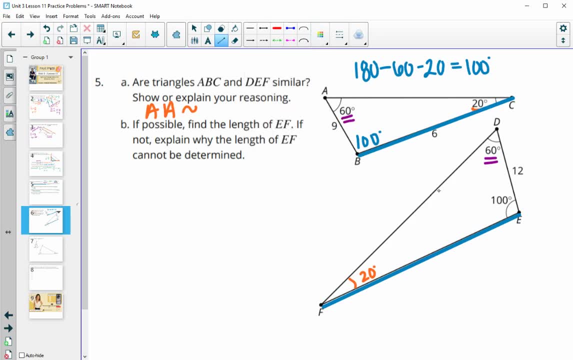 So then we have to look for another set of similar sides and hope that they both have side length measures. So this triangle, the 12 connects the 60 and the 100. And in this triangle, the nine connects the 60 and the 100. 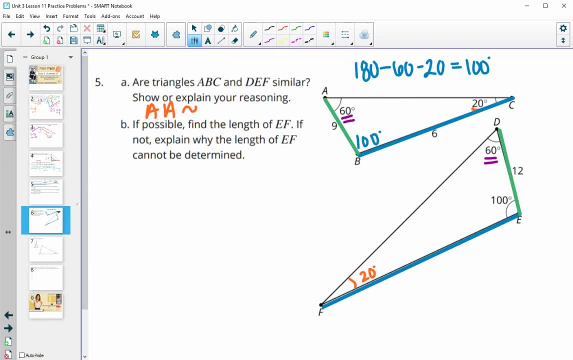 So that means we're going to be able to find the missing length. So you've got a couple of ways to find the missing length, A couple of ways you can do this. OK, you can figure out. So now we're missing this measurement here, right in this triangle. 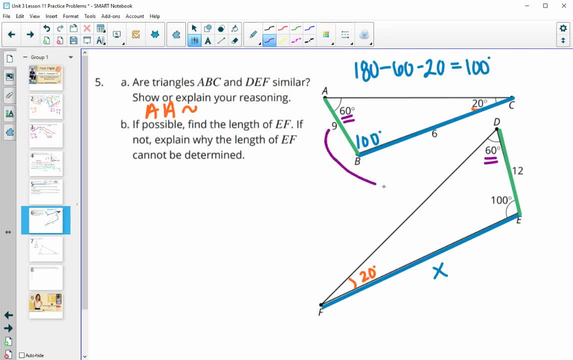 So you can figure out. what number do I multiply nine by to get 12.. So you can come up with the scale factor. And so you can do that by doing nine Divided by 12.. OK, so that'll give us our scale factor, is not? 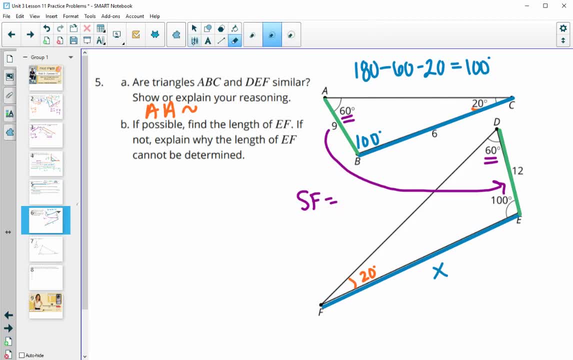 Sorry, 12 over nine. OK, so taking 12 divided by nine, And so then that reduces to four thirds. So then you could do the same thing with the six. OK, to get to the X. So we can do six times the scale factor of four thirds. 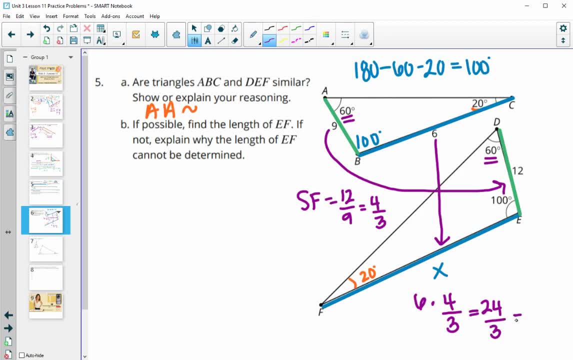 So that's going to be 24 over three, which is eight. So then side EF is going to equal eight. Another way that you can do that is By doing proportions, So then you can set up. I like to start with the missing one. 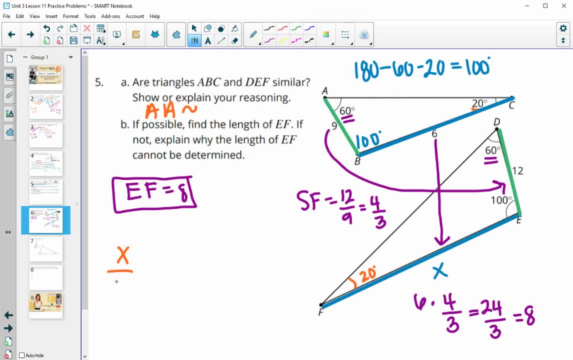 So I'm going to compare X to its corresponding side of six by putting it in a ratio: So X divided by six, And I know that's going to equal 12 divided by its corresponding side of nine, And then you can cross multiply here. 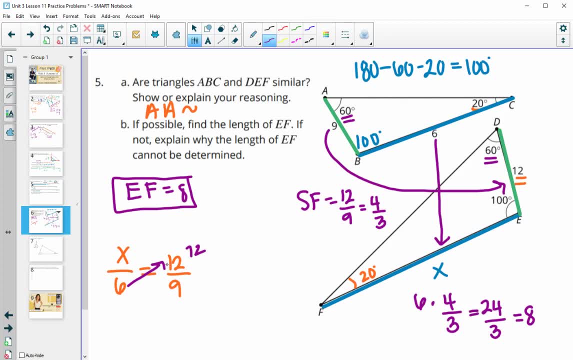 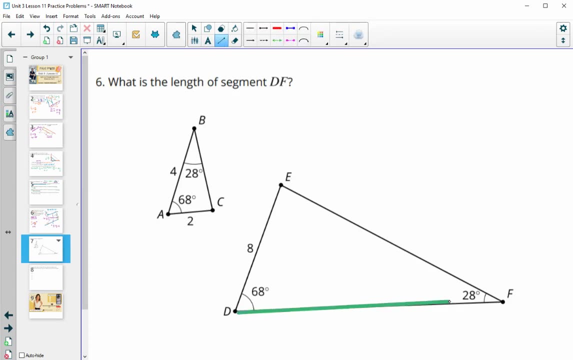 So six times 12, which is 72 divided by nine, which again gives you that eight. So either That way is fine to find the missing length, Number six, what's the length of DF? So here's side DF, Again, we'll compare that in the other triangle, the 68 and the 28.. 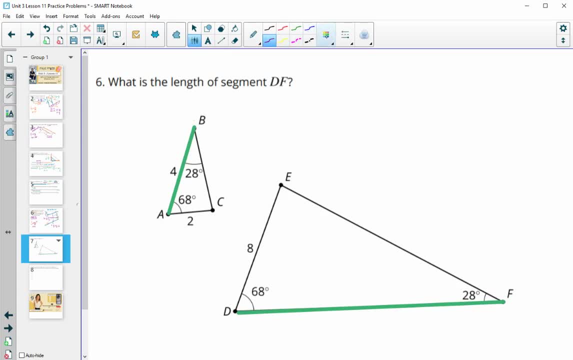 And if you're not using colors like this, you're not kind of highlighting the sides. I sometimes like to use dots, So then I'll just put a dot on the sides that are the same And then on the next one that I'm comparing. 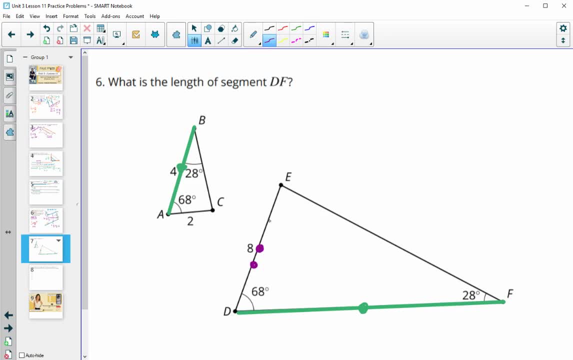 So now I'll put two dots to compare. So this is the one that's touching the 68 degree angle, That's going to go to this one, So that it just helps me kind of keep things straight. So if you're not using colors and you're just using a pencil, if you wanted to use dots, that might be a good option. 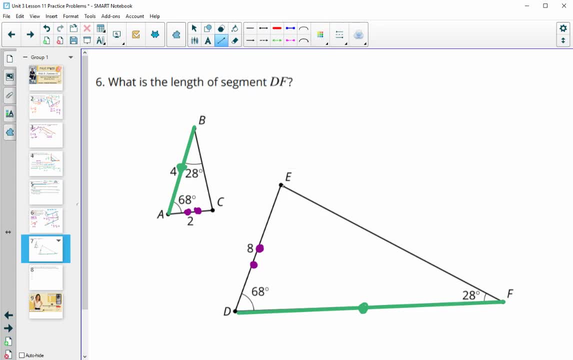 But I am going to put the color on here. So then DE compares to AC. So again, multiple ways To figure this one out. if you're using scale factor, if we look at comparing the two purple sides, we see that we just multiply by four to get from two to eight. 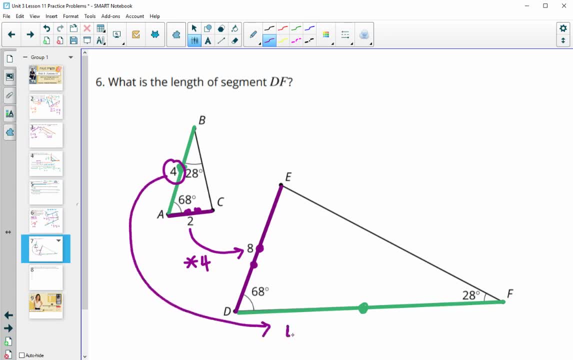 So then we're going to do that with this other side to get this one. So then four, the original side, times the scale factor of four, gives us 16. for side DF. Again, you can also set up proportions. So then if I just called this side X, that side compares to the four. 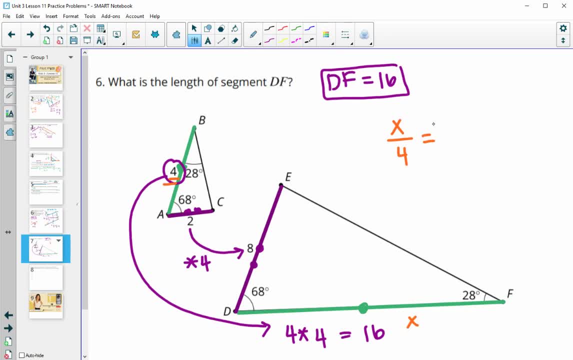 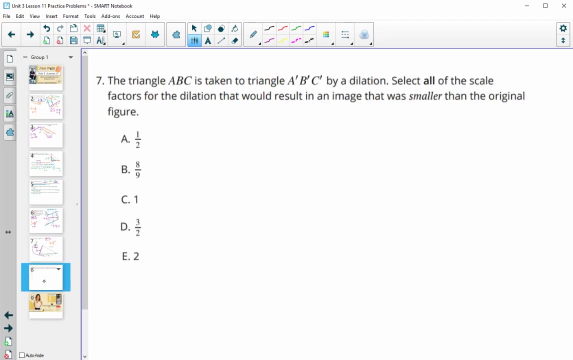 So X over four should equal eight over two, And then cross, multiply and divide. So four times eight is 32.. Divided by two gives you 16 as well. All right, Then. number seven says triangle ABC is taken to A, prime B, prime C.